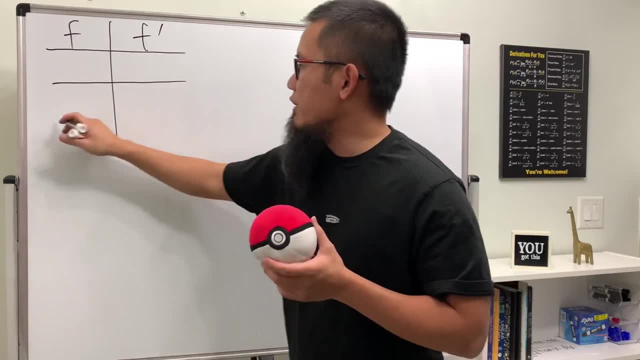 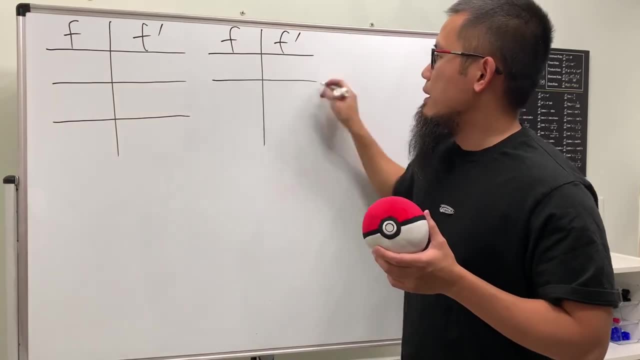 So we have f and f prime and right here I'm going to give you guys three first and then another table right here with the other three. And keep in mind of the order of the functions that we put in, because if you put it down in this, 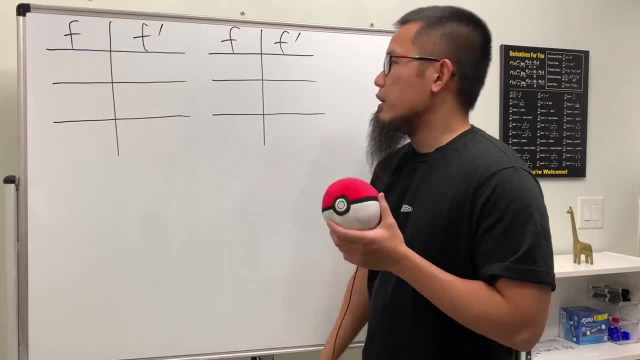 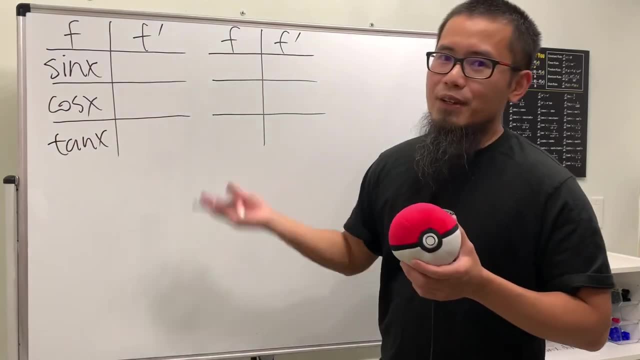 order. I think the pattern is easier to remember, So I'm going to start off by putting down sine x right here, and then cosine x and then tangent x- Yeah, the first three trig functions that we learn right. and also sine over cosine gives us tangent. That's pretty cool. 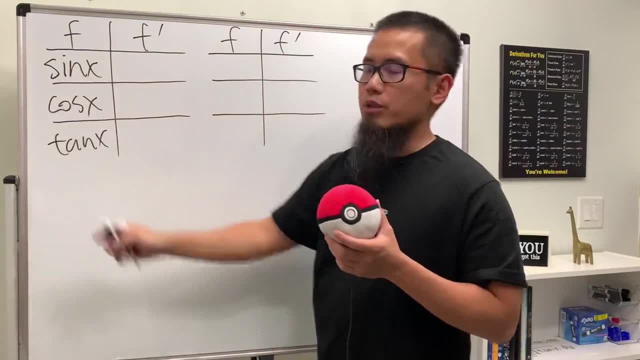 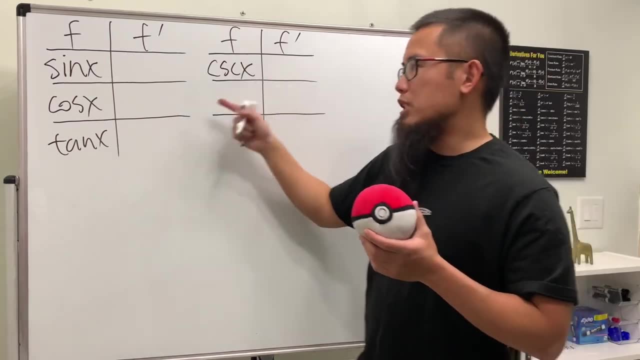 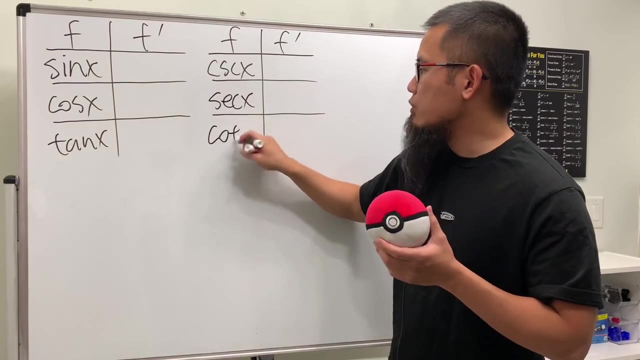 And right here we will be putting down the reciprocals. so this is going to be the reciprocal of sine x, which is called secant x, and this is going to be the reciprocal of cosine x, which is the one over cosine x. And that's the secant x, and this is one over tangent x, which is called tangent x. 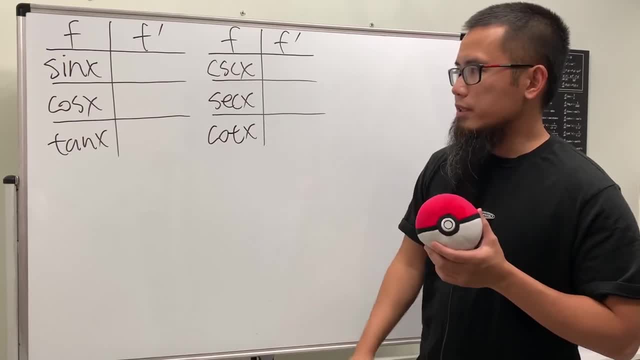 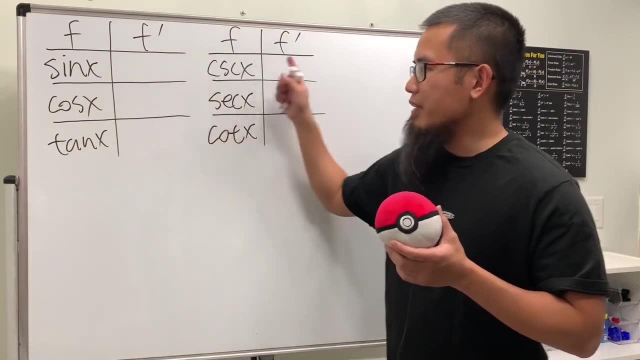 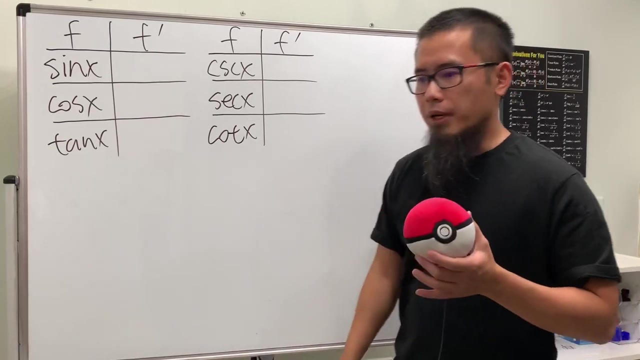 All right, and here we go. First, notice that we have three core functions. They all start with a, c, and I will tell you guys this right now: They all have negative derivatives, so that's how you can remember which one has negative, which one has the positive derivative. Okay, to figure out this. 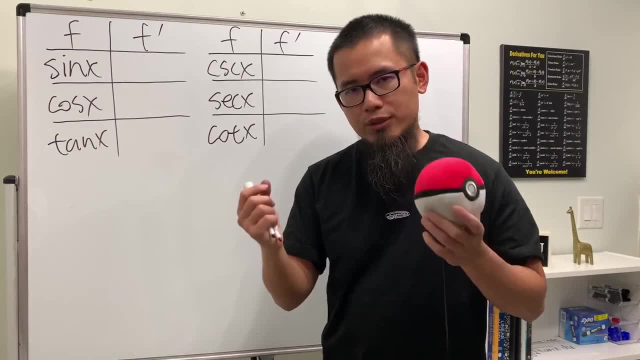 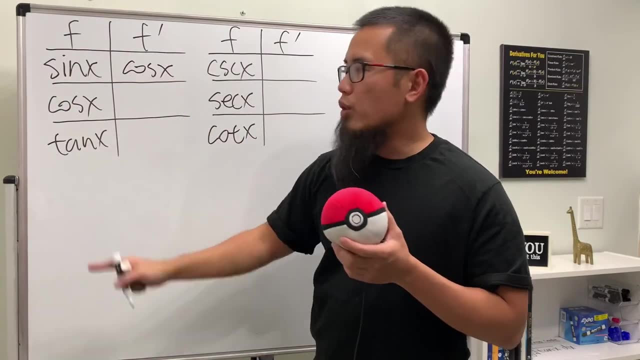 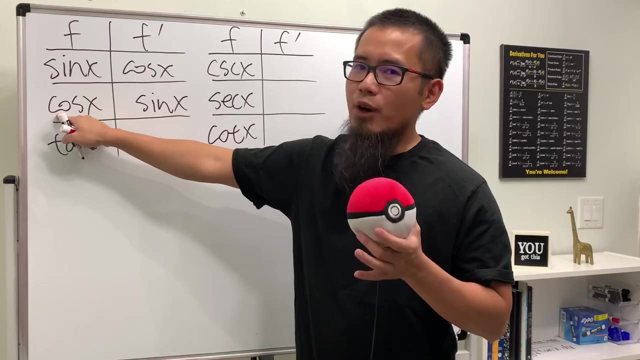 and that you have to remember that sine and cosine, they are better than the negative one. friends, in calculus the derivative of sine x is cosine x and the derivative of cosine x is sine x. but remember what we said earlier: co functions, any function. so it's a c right here. 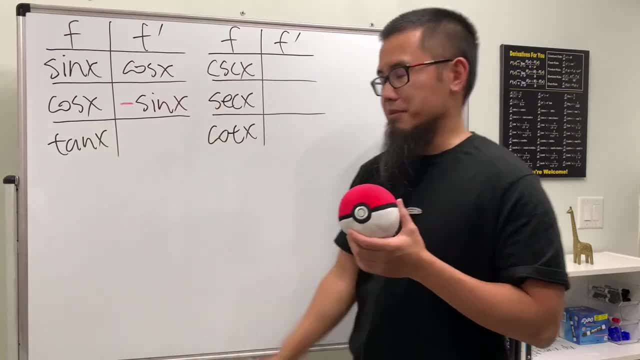 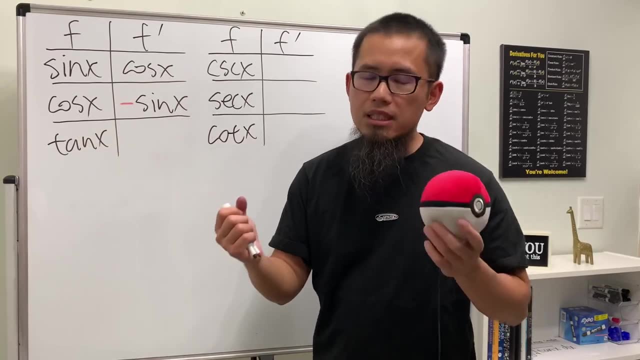 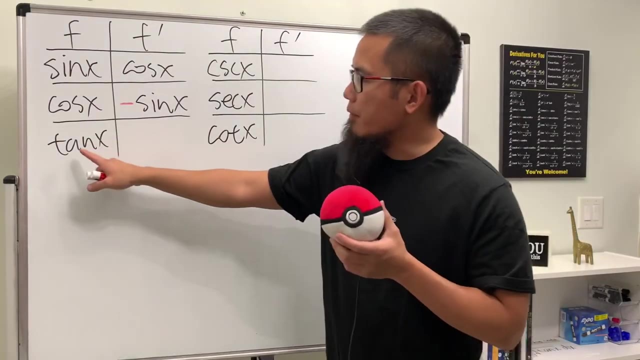 we'll have negative derivative, so we have negative x, right cool. now next, maybe we can figure out tangent, and i will tell you tangent and secant, they are best friends in calculus as well. for this, right here i will tell you: the derivative of tangent x is secant square x. so just remember. 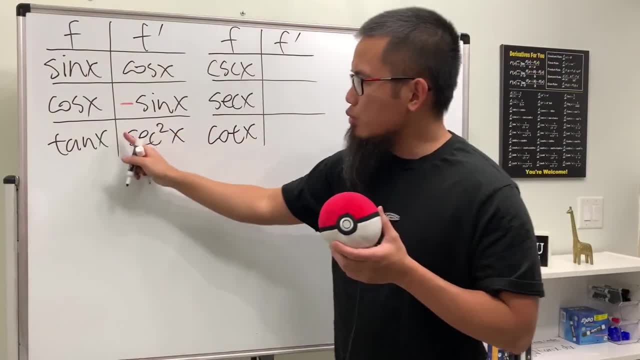 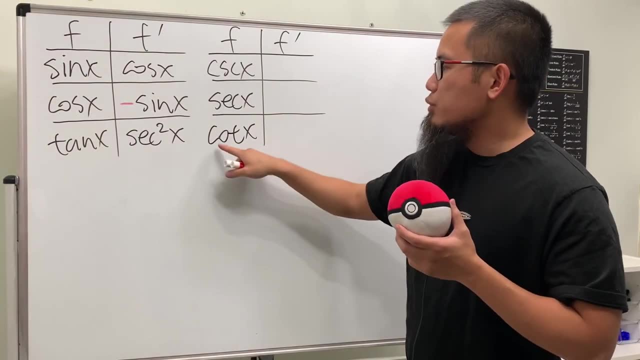 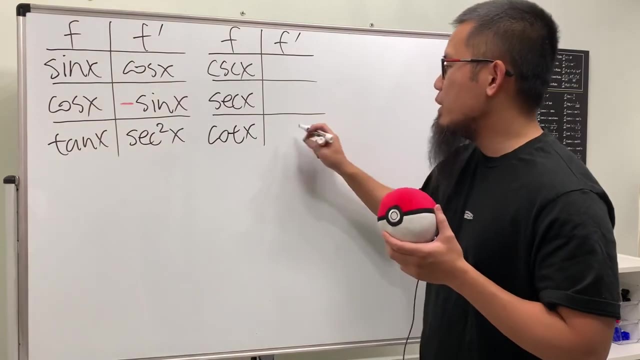 the second power. right here, and you know, once you remember this, you also can kind of reason out for the derivative for cotangent x, because you see, this right here is the co-function of tangent, so right here it will be the co-function for secant, namely we get cosicat and also the square. 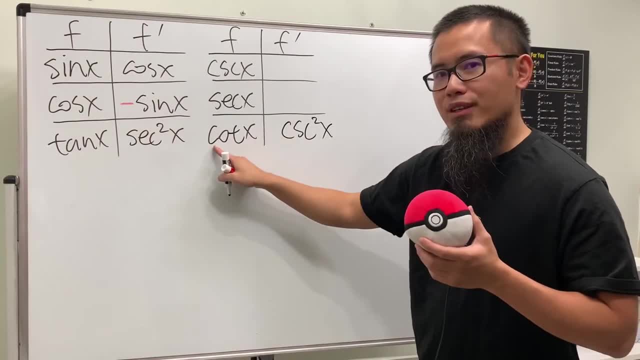 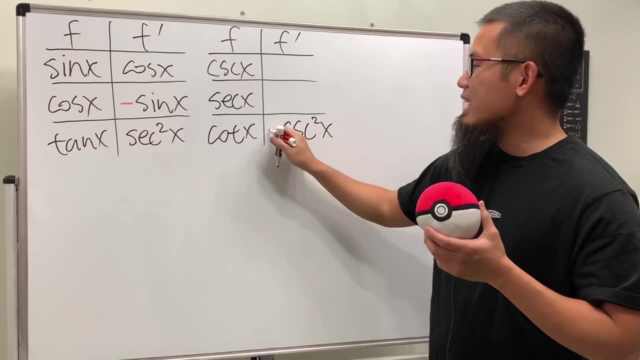 right here, so we can get the co-function for secant and also the square right here. but remember, here we have co-function right. this function starts with a, c, so we will have negative derivative. so the derivative of cotangent x is negative. cosecant square: yeah, okay. so now we just 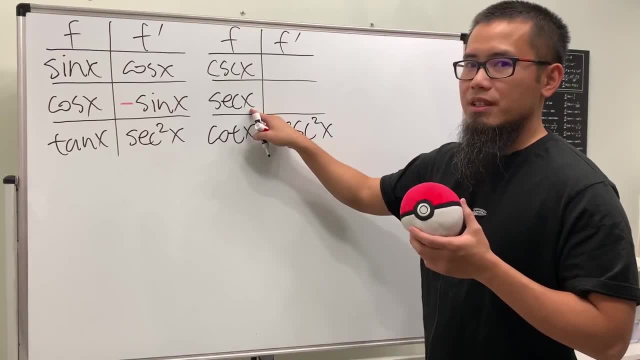 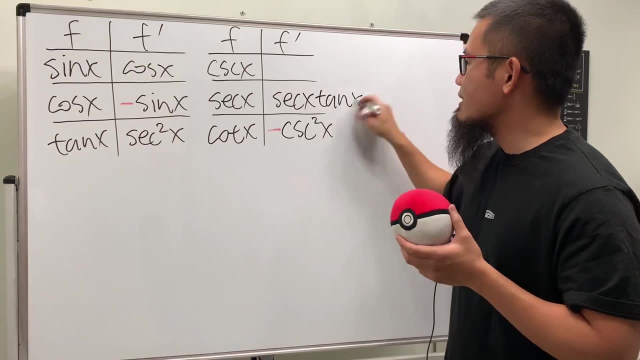 have to figure out this too well. we can do secant x first. i will tell you secant repeat first, and then don't forget to multiply by its best friend, which is tangent x. so the derivative of secant x is secant x. tangent x. so the derivative of secant x is secant x. tangent x. so the derivative of secant x. 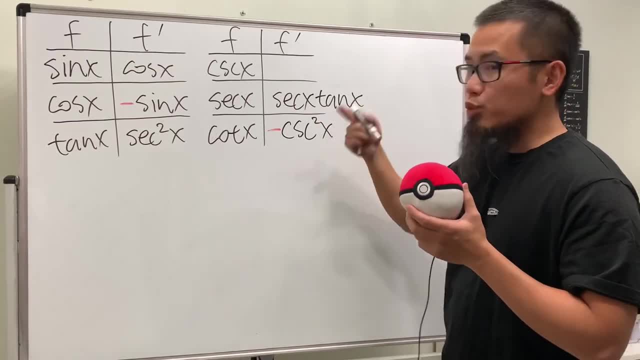 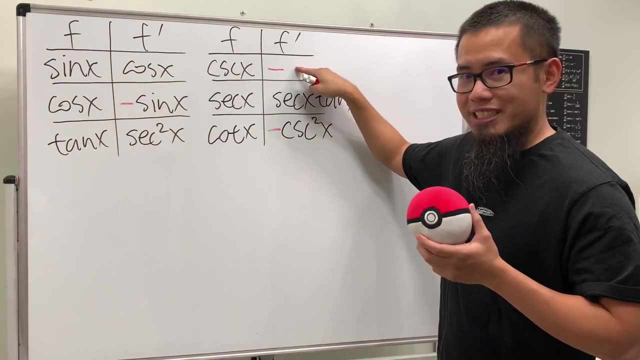 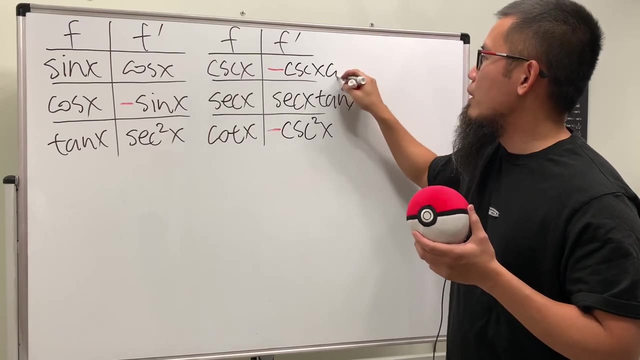 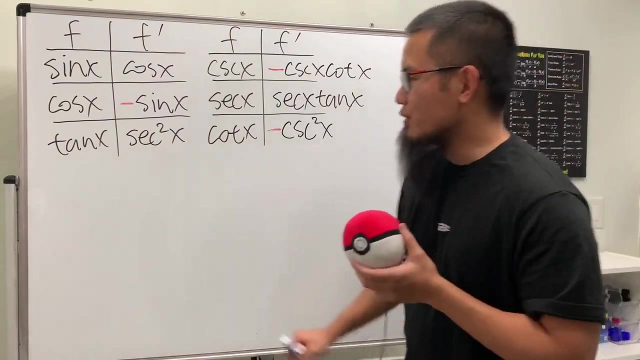 and once you have this again, you can kind of reason out. for cosecant x, yes, it's going to be negative, and then we will have cosecant x repeat, and then we will have to multiply by cotangent x and we're done. yep, so that's it. and now let's talk about the inverse trig functions. and again, 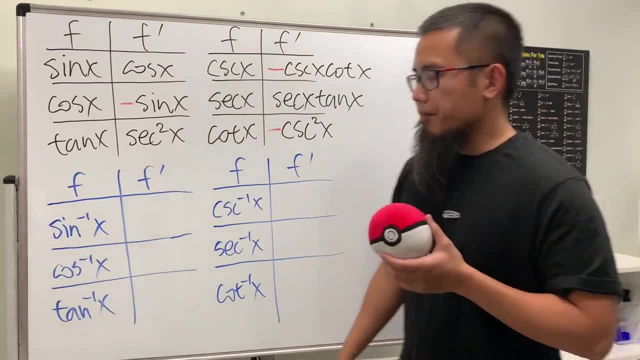 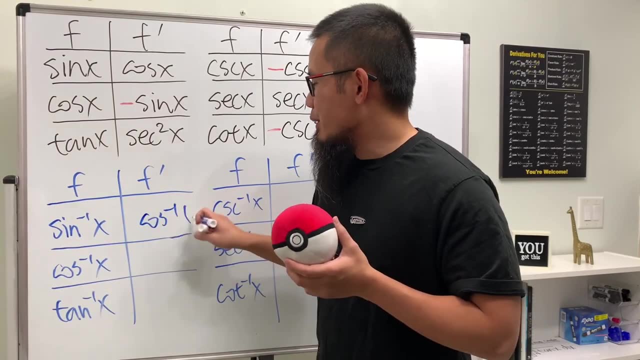 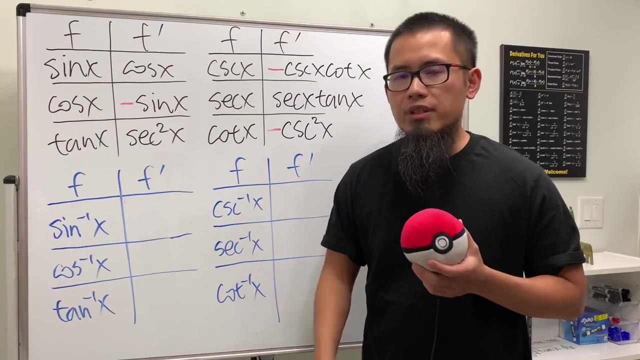 i'm just going to put them down right here for you guys. okay, fortunately, the derivative of inverse secant x is not inverse cosecant x. no, this is not correct. okay, so don't do that. and this right here takes some time to remember, so be sure you put in the 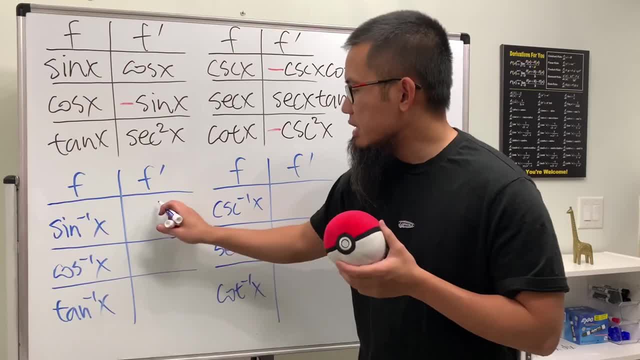 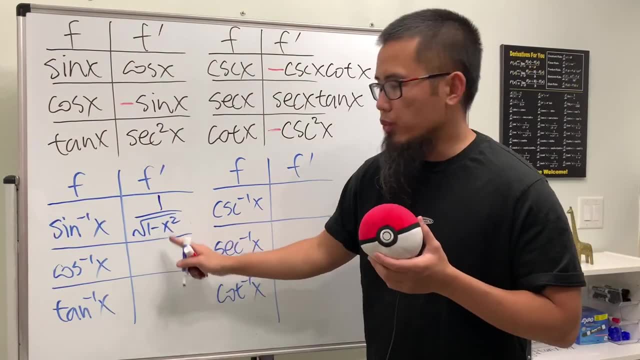 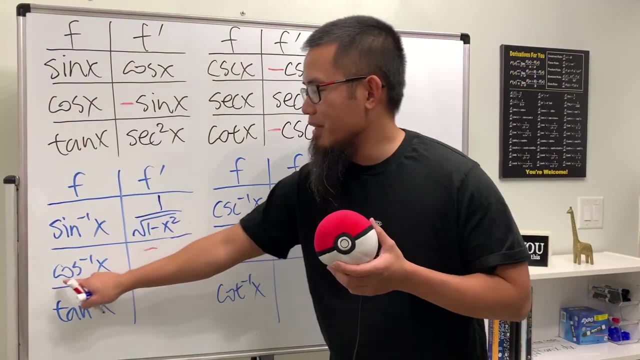 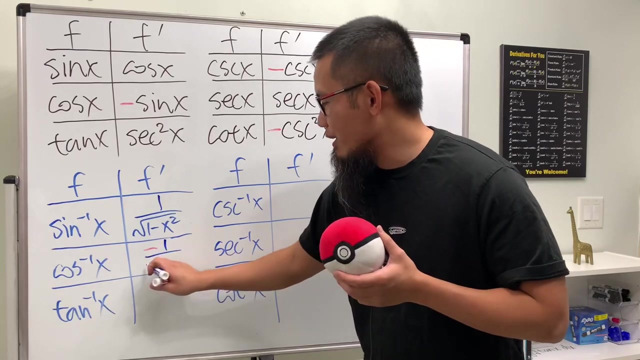 efforts for them. first, the derivative of inverse secant x is 1 over square root of 1 minus x square. and if you remember this, i will tell you. you know the derivative for inverse cosecant x for free. first it's going to be negative because it has a c right. and then let me tell you. you just write this down: 1 over square root of 1. 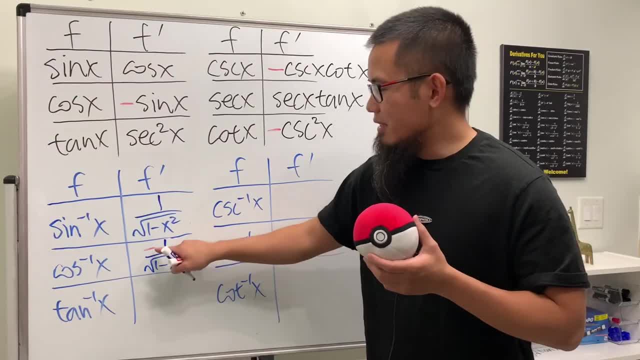 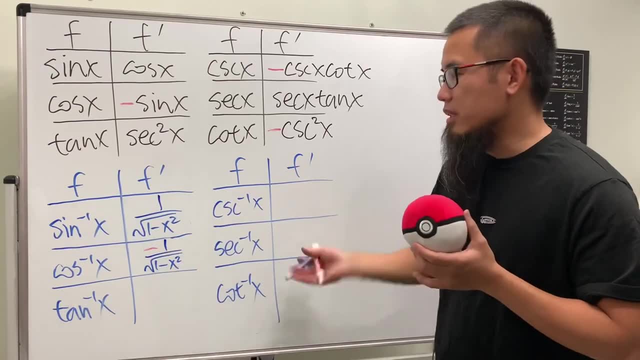 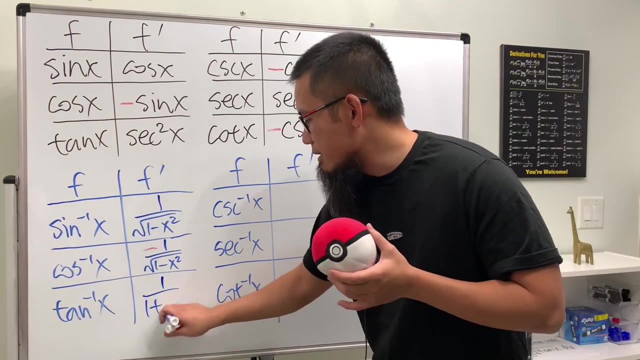 minus x squared. you see how similar they are. this is just a negative version of that. that's all yeah, and you guys can check out my other video for the reason for that. but here again, it's just how we remember the derivatives. perhaps next we can talk about the inverse tangent. we will get 1 over 1 plus. 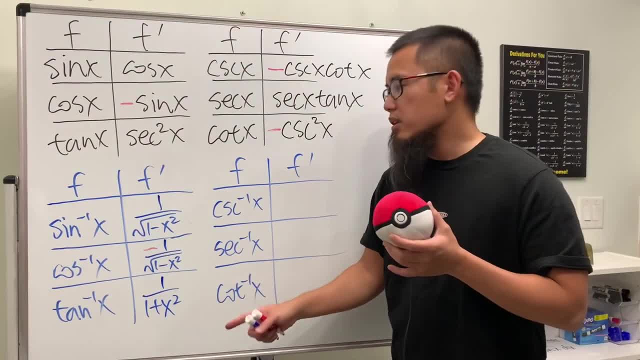 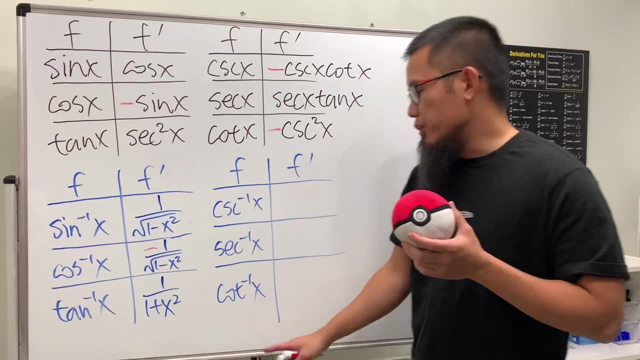 x squared, and i can tell you, in calculus 2 in particular, this and that are very common, so be sure you remember them really well and you know, once you have the inverse tangent, you know the inverse cotangent for free, because it's just going to be. 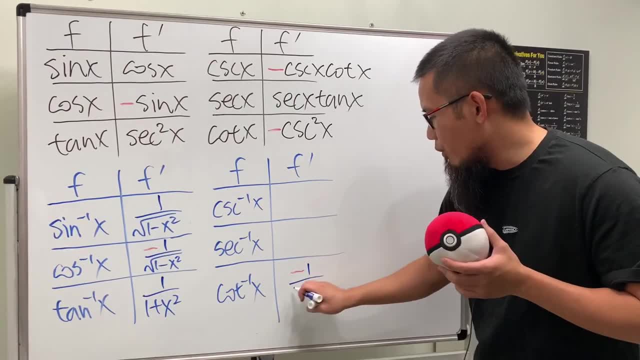 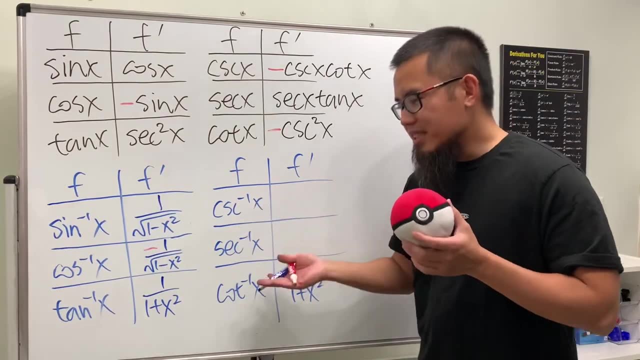 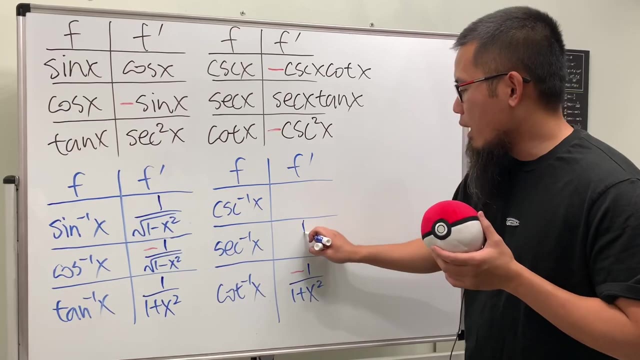 the negative of that. so negative. 1 over 1 plus x squared, and then we are done for that. okay, for inverse secant and inverse cosecant. they are not so common, but here's their derivatives. for the inverse secant, we get 1 over x times the square root of 1 minus x squared, and then we are done for that. 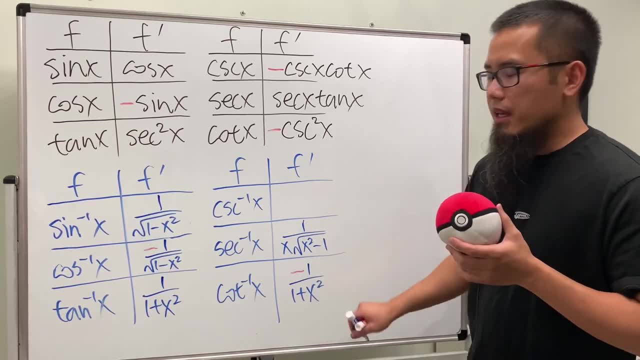 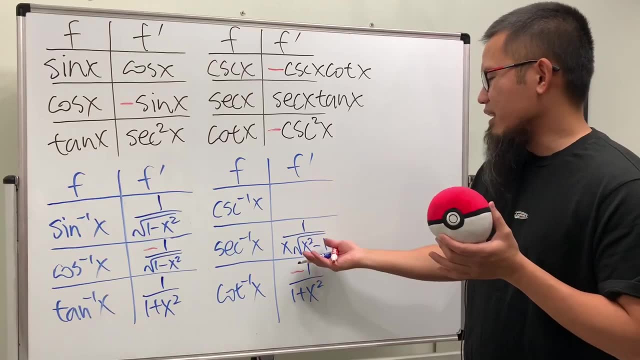 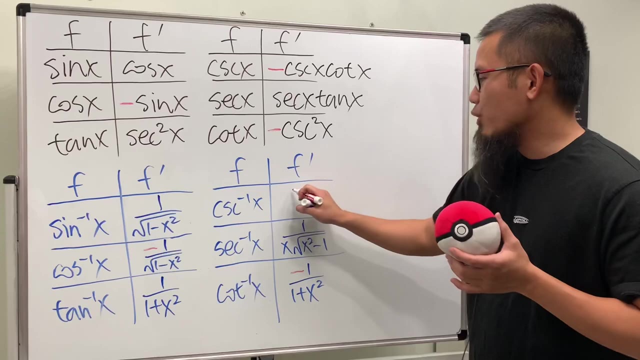 square root of x squared minus 1, and some people might put an absolute value right here. it really depends on the domain that they pick, but if you write it down like this on my exam, that's totally okay, and once you remember this, you know this for free. yes, it's going to be negative of that. 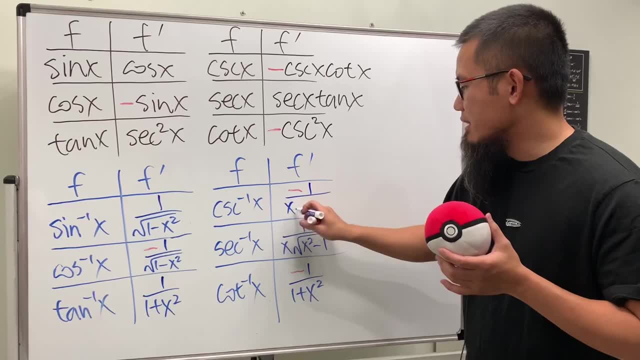 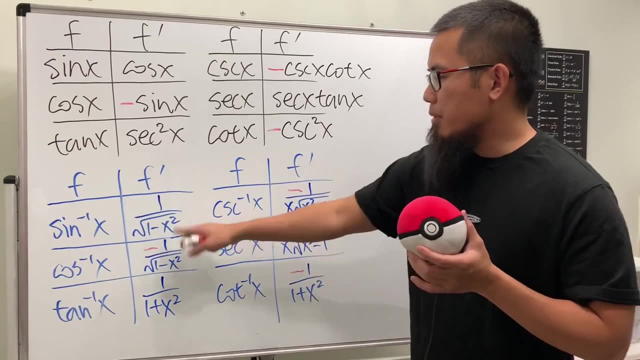 so we have negative 1 over x times the square root of x squared, minus 1. and you might be wondering how can we remember if it's a plus or minus x squared, and then we are done for that. so we are done for that. so if it's a plus or minus in between of the 1 and the x squared and things like that, i can tell you. 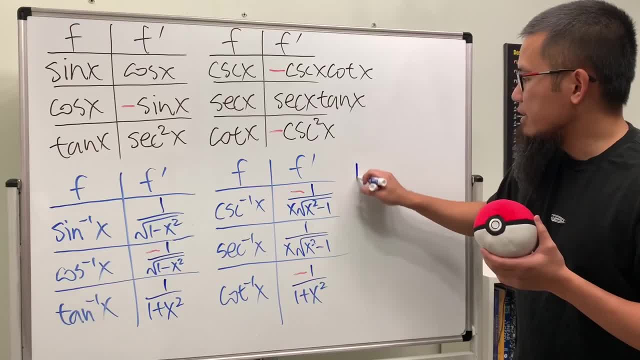 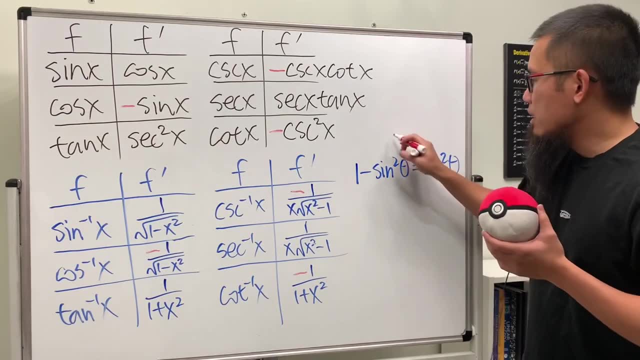 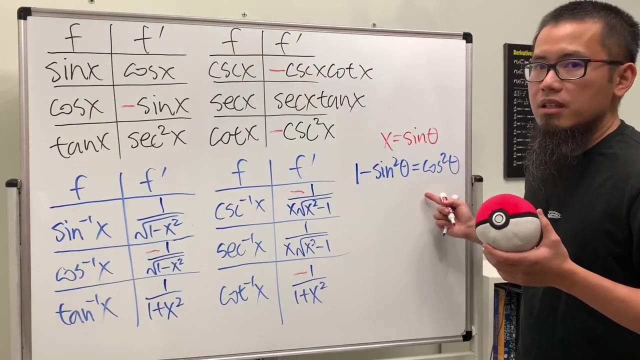 for the inverse, sin x. we look at this identity, 1 minus sin squared theta being equal to cosine squared theta, and you see x equals sin theta. that's exactly what we will get right here and this is the identity. and if you guys remember the proof that, how we get from here to there. 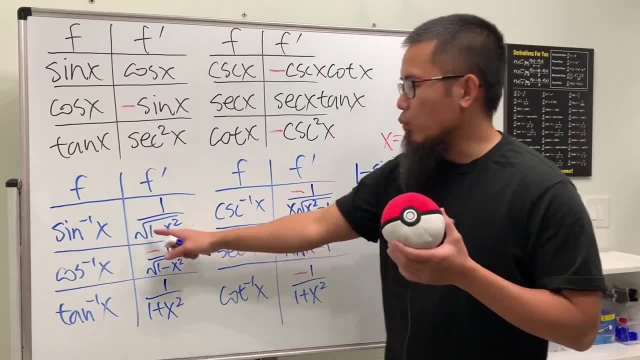 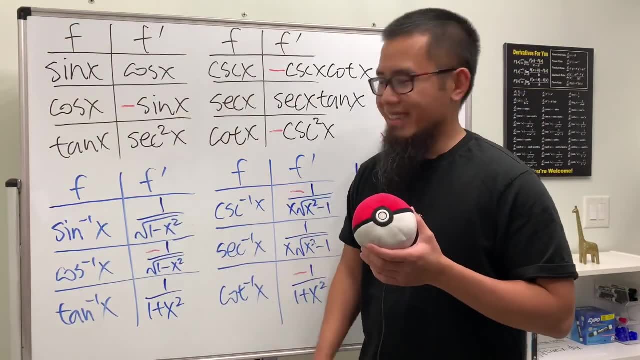 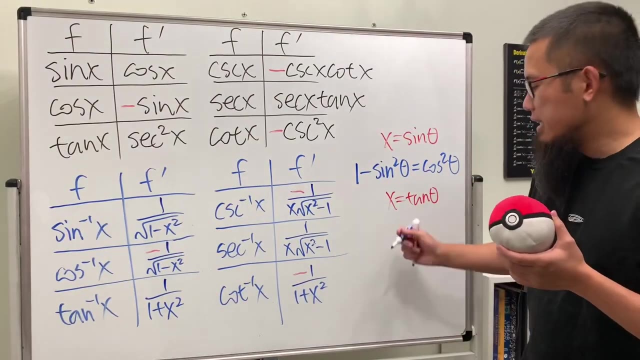 this is the identity that we use. so that's why we have the 1 minus x squared and this is the square inside of the square root, on the bottom. and again, if you know this, you know that for free. next, for inverse tangent: well, if you let x equal tangent x, then you can look at the identity. 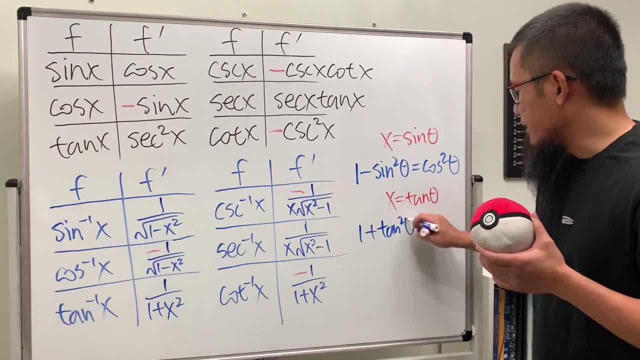 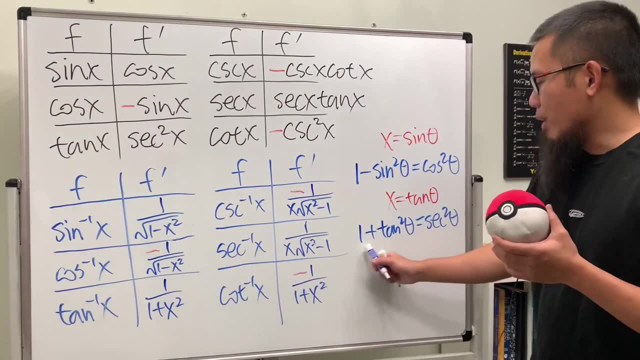 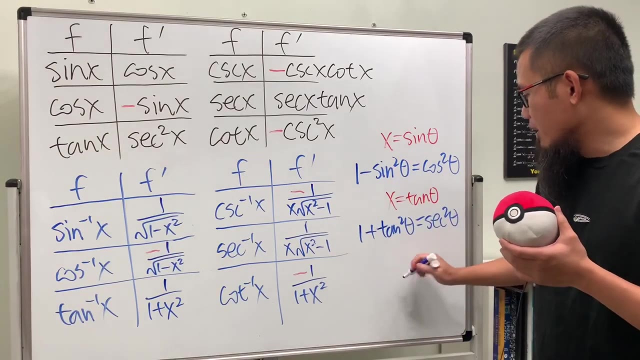 1 plus tangent square theta. this right here gives us secant square theta. so that's why we have the 1 plus x square, 1 plus tangent square on the bottom right here, right. and lastly, let's talk about the inverse secant. of course, that would be just: you move the 1 to the other side and you can.